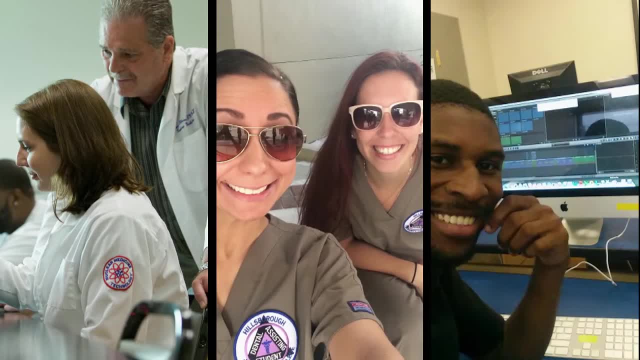 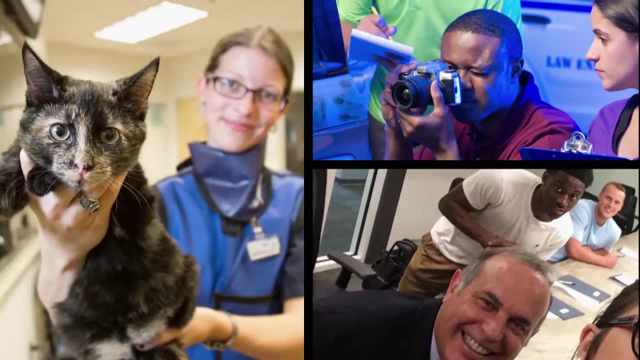 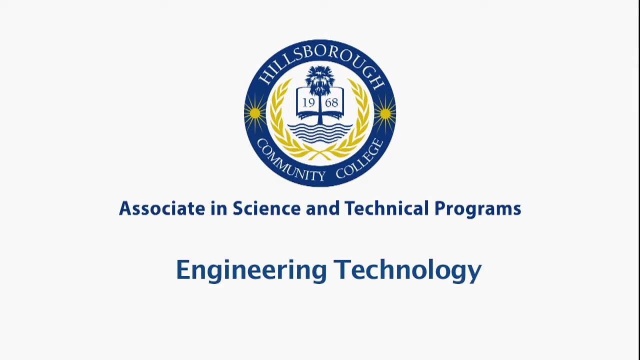 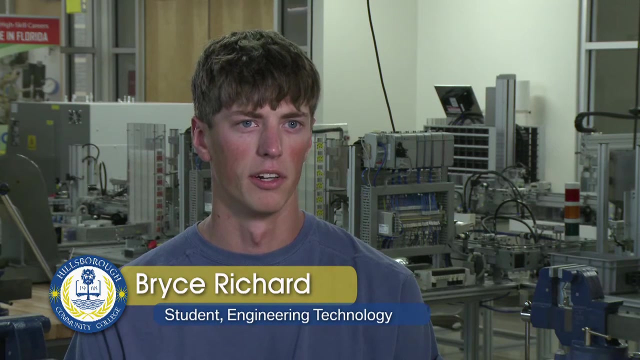 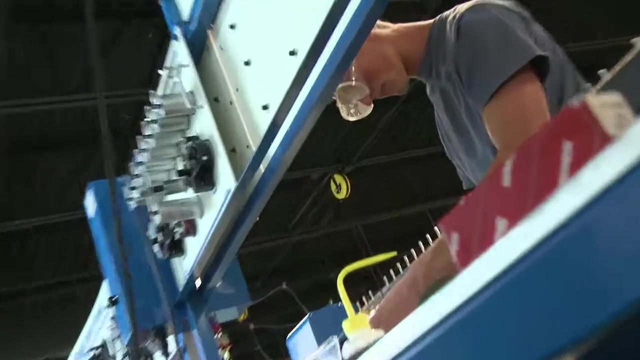 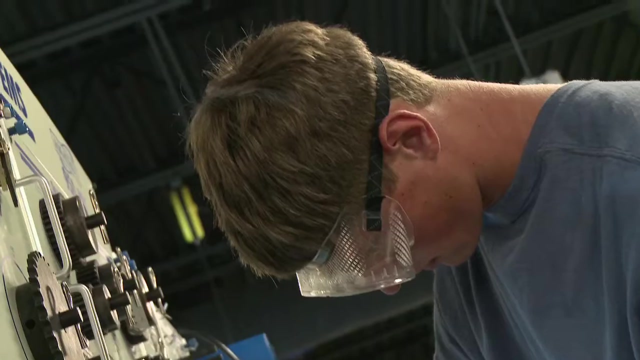 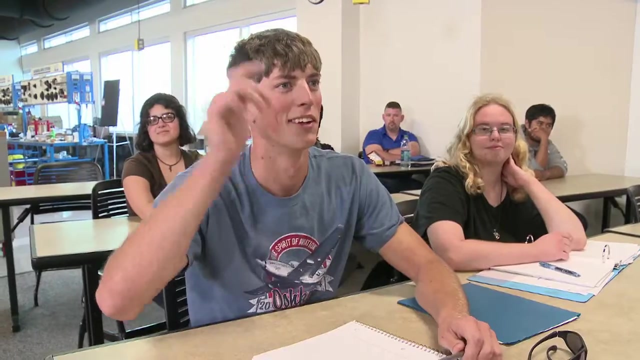 I'm in the engineering technology program for advanced manufacturing and we focus on everything from motors and controls to industrial maintenance. I didn't think traditional engineering was where I wanted to go. I wanted to be more in the field and work with my hands, along with other technicians, and this program can. 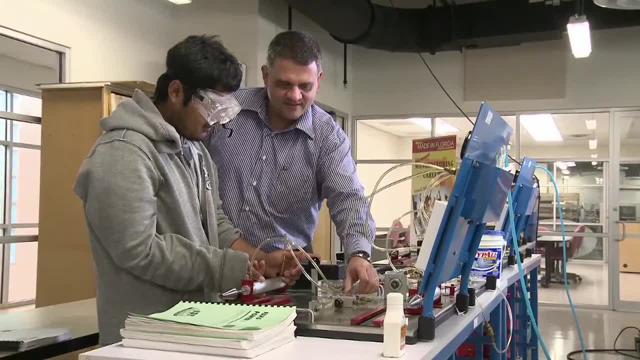 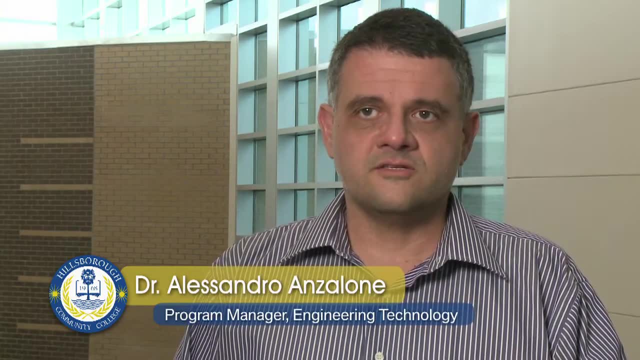 lead to management, which is something I'm interested in. In our program we prepare manufacturing technicians. Students get an associate of science in engineering technology. They get several certifications at the same time and they get a job. I think the only time we really even sit down in our chairs in the classroom is the first. 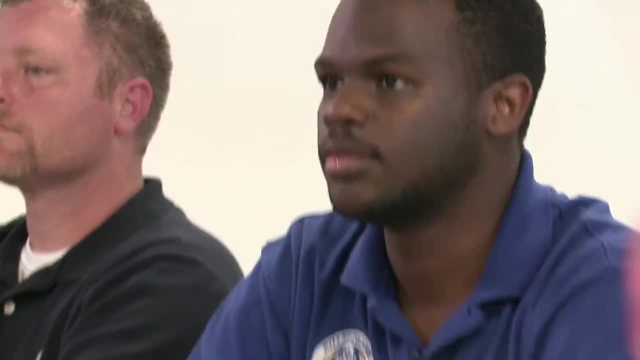 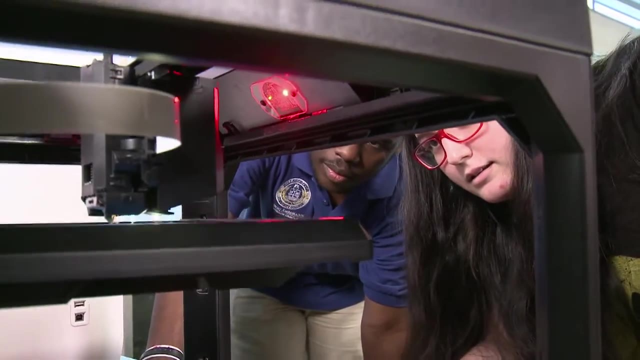 day of the class, just as an introduction, and then we're working by ourselves on the hardware and the software, programming the logic to control different processes. It's really a fun group of people here, People that like more the hands-on or the applied aspect of technology. That is my perfect. 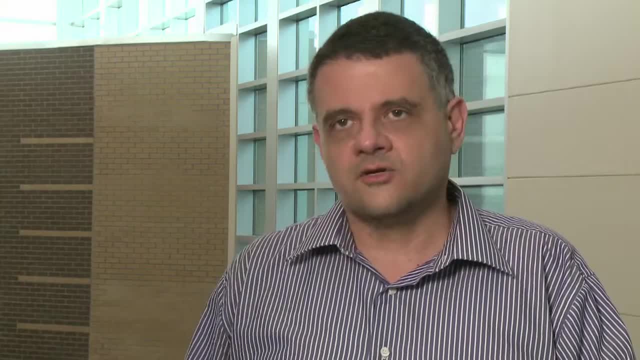 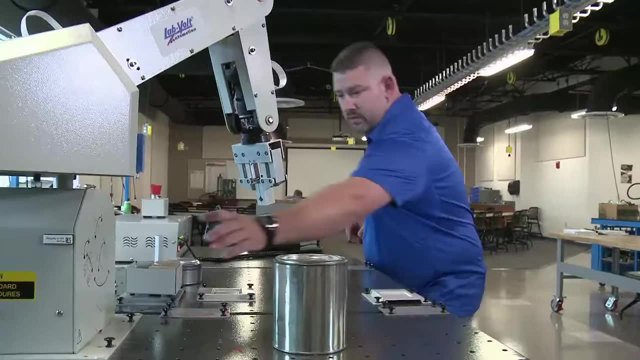 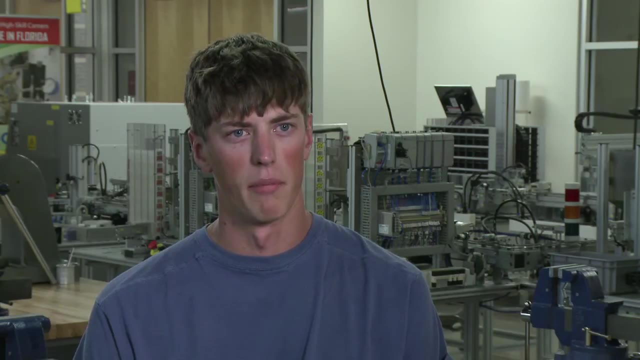 student. We have motors and controls, hydraulics. We have 3D printers, We have mechanical drive systems, So a wide variety of instruments and equipment used in manufacturing, Most of which is real life components. I'll complete my degree in May. I almost wish I wasn't completing it yet because we just 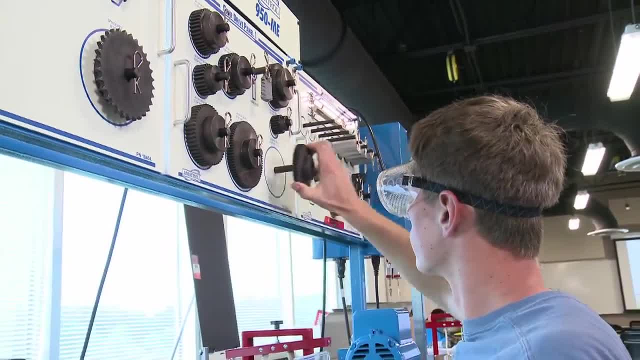 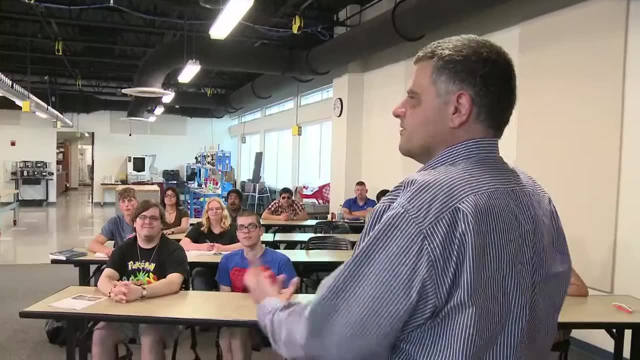 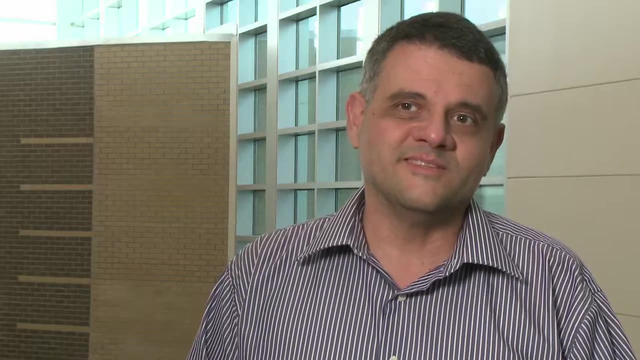 keep getting better and better tools. This program is going to just keep advancing to prepare you even more so for the job market. Normally I can get people that are coming at eight dollars an hour and in one year they are at twenty-eight dollars. That is my favorite thing: Changing people's lives. That's why I do what I do. 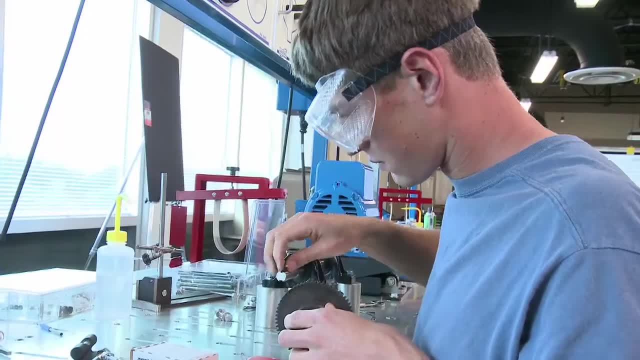 I've had multiple job offers here even before I've completed my degree, and when you get your job offer and you're sitting down in an interview and it's pretty clear that they want you, that's when you know you made the right choice.